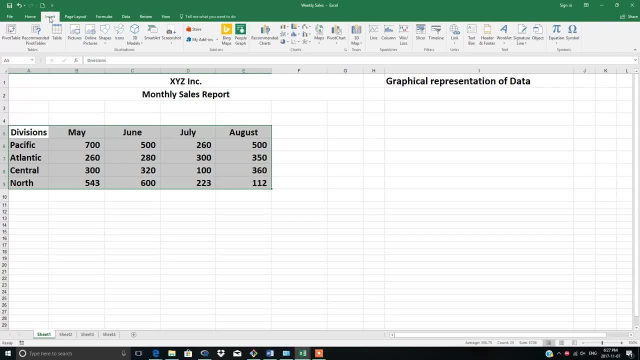 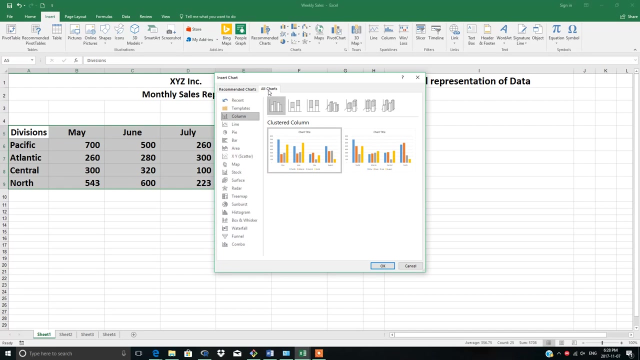 select your data and then go to the insert tab. In the insert tab you will see the charts group. In charts group you have pie chart, line chart, bar chart and different kind of charts are here. If you are not sure which chart you are looking for, so just click the recommended chart here and all charts. So 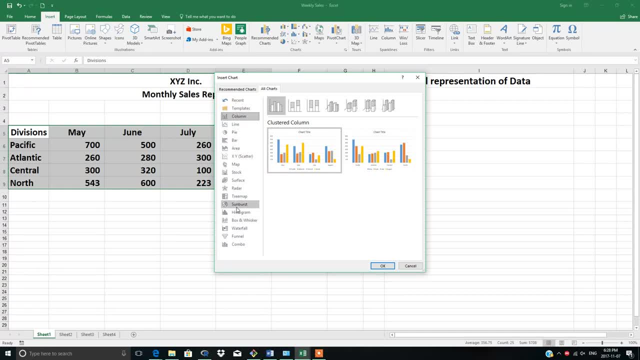 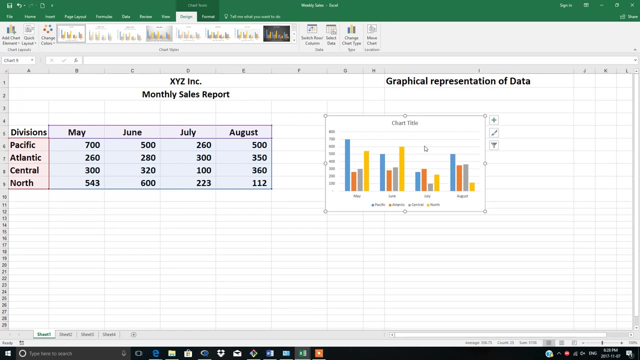 you will see the line chart pie chart, bar area and so on. Suppose, in this case we are looking for the clustered column, So this is the clustered column, So you can move your chart here. So see in the chart, this is the chart title. if you want, you can write down or you can. 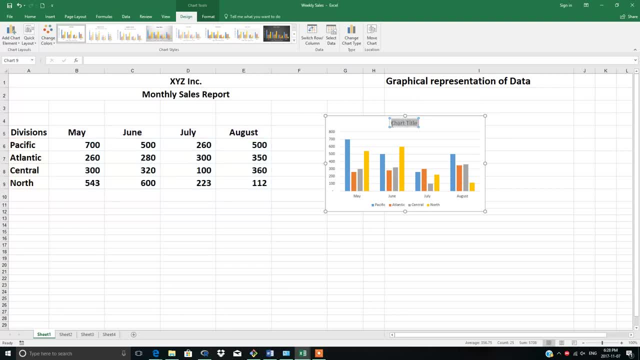 change the name of your here. Suppose this is the XYZ company. You can write down here: XYZ Inc. This is called the legend Means. the blue represents the Pacific, orange represents the Atlantic, grey central and yellow represents the north. and these are the filter button, suppose, if you do not want to show your audience all the Pacific. 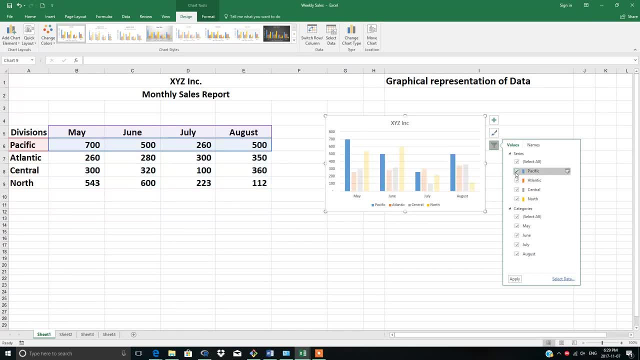 Atlantic, central and north. you want to show only the Pacific and the north, so you can just remove this check mark and apply so you can see only the Pacific and north are there. if you want to bring back open this and apply similarly, this color is style, this is the style and color. if you do not want this color, so 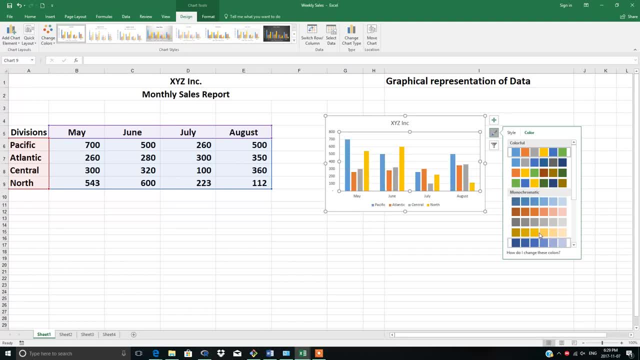 you can change the color. these are the different colors available here, whatever you like. and then this is the plus sign: open this. and then this is the plus sign: open this. and then this is the plus sign: open this. and here you will see: the legend is check mark. it means our legend is here. 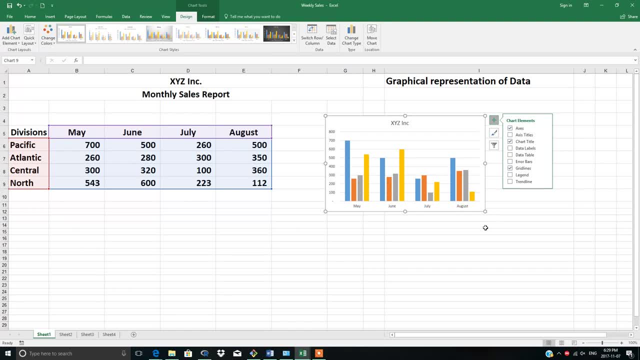 if you do not want your legend here, just remove this check mark and see it's gone. if you want to bring back here and then data levels, if I click here, you will see these amounts will come on the top of each graph. if you want data, table here. 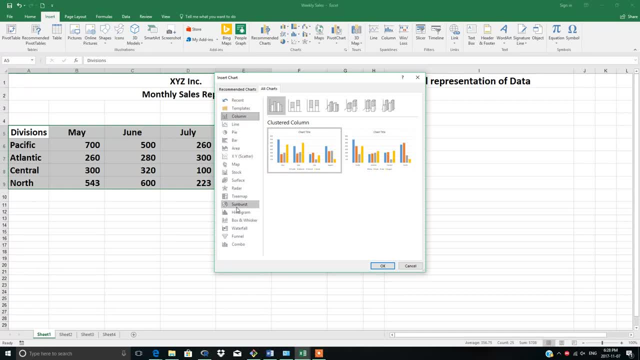 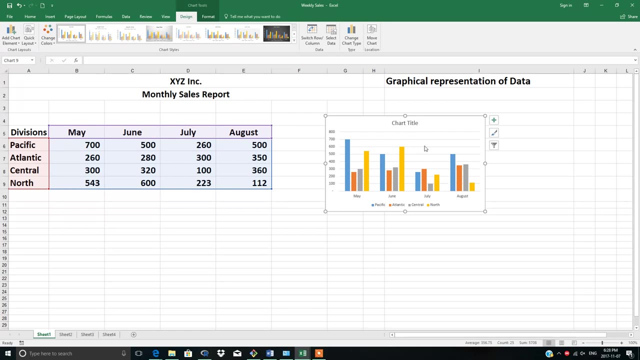 you will see the line chart pie chart, bar area and so on. Suppose in this case we are looking for the clustered column. So this is the clustered column. Then click OK So you can move your chart here. See, this is the chart title. if you want, you can write or change the name of your chart. 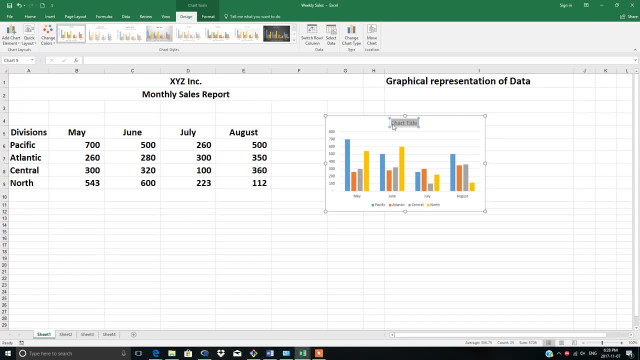 here Suppose. the chart title is XYZ INK. This chart is called legend Means the blue represents the Pacific, Orange represents North, Blue represents the West, Yellow represents the North, Brown represents the South, the Atlantic, grey, central and yellow represents the north. and these are the. 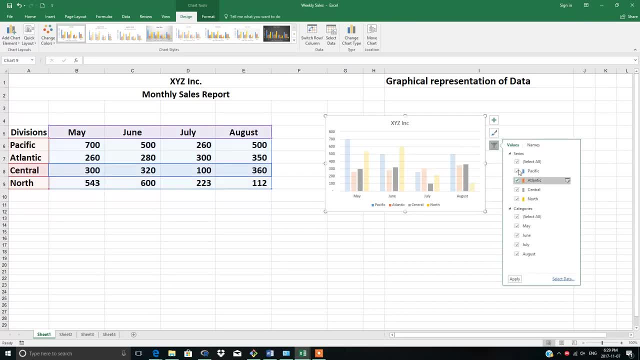 filter button. suppose if you do not want to show your audience all the Pacific, Atlantic, central and north, you want to show only the Pacific and the north. so you can just remove this check mark and apply so you can see only the Pacific and north are there. if you want to bring back open this and apply similarly this, 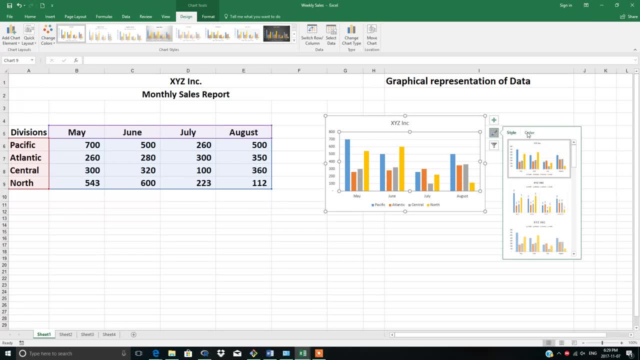 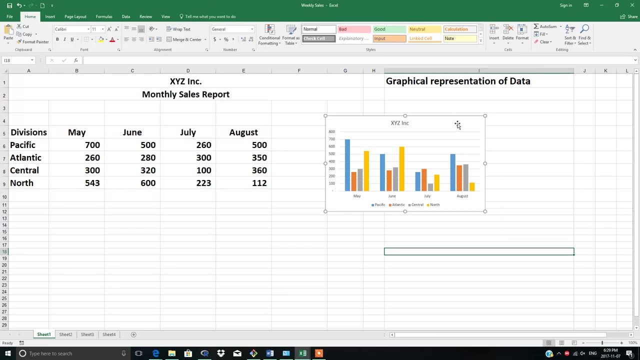 color is style. this is the style and color. if you do not want this color, so you can change the color. these are the different colors available here, whatever you like. and then this is the plus sign: open this. and then this is the plus sign: open this. and then this is the plus sign: open this. 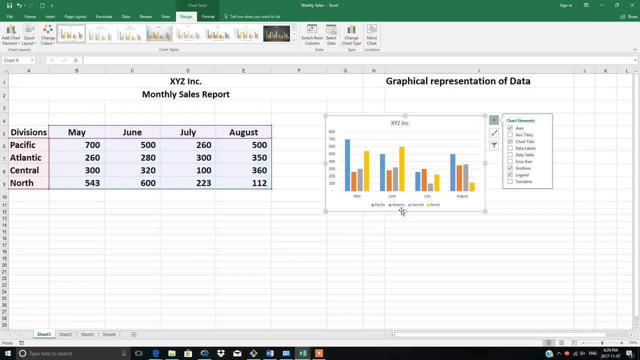 and here you will see. the legend is check mark. it means our legend is here. if you do not want your legend here, just remove this check mark and see it's gone. if you want to bring back here and then data levels, if I click here you will see. 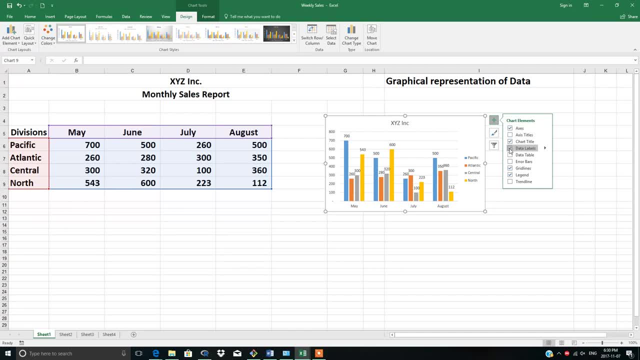 these amounts will come on the top of each graph. if you want data table here, then you will see. the amounts are here. if you will change these amounts in future- suppose in July you want to make it 500, so you will see the change here on your graph as well. see the blue one and then this is the.